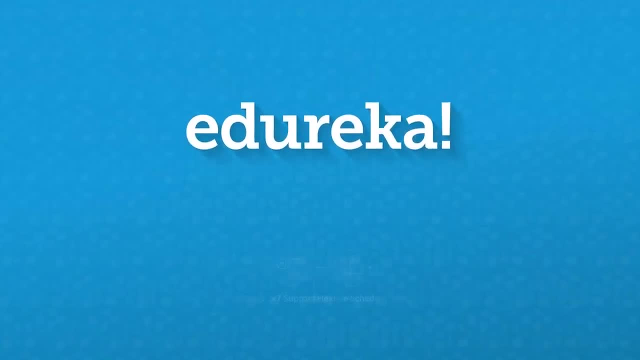 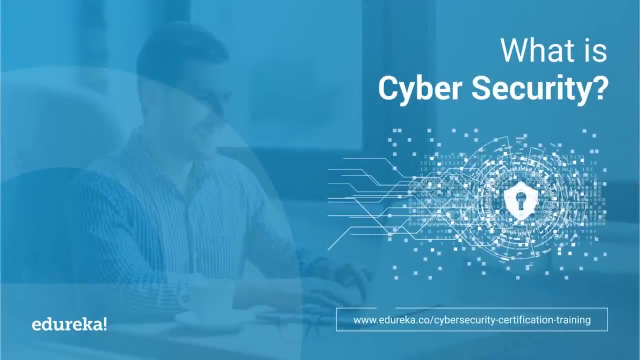 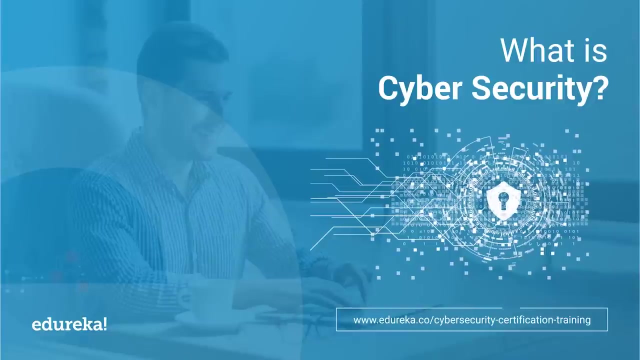 It can be rightfully said that today's generation lives on the internet and we general users are almost ignorant as to how those random bits of ones and zeros reach securely to our computer. It's not magic, it's work and sweat that makes sure that your packets reach to you unsniffed. 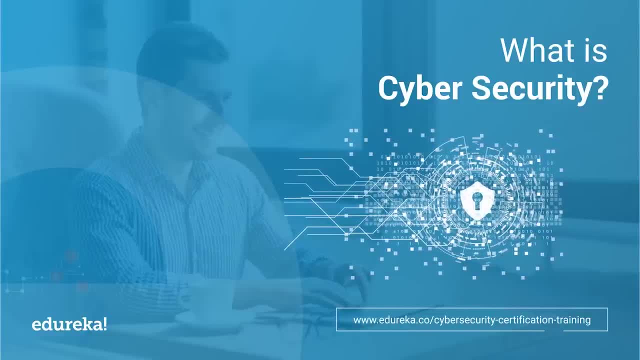 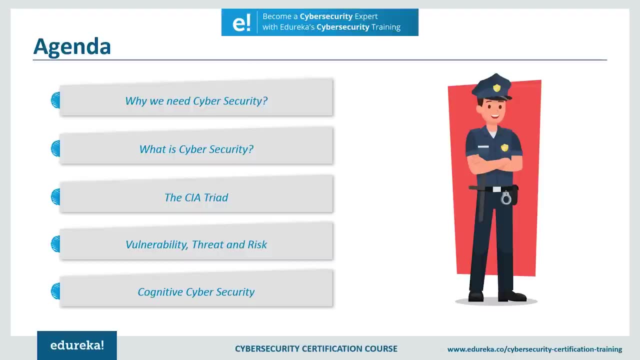 Today I, Arya Paul from Edureka. I'm here to tell you guys about how cyber security makes this all possible. Now, before we begin, let me brief you all about the topics that we're going to cover today. So, basically, we're going to ask three questions that are important to 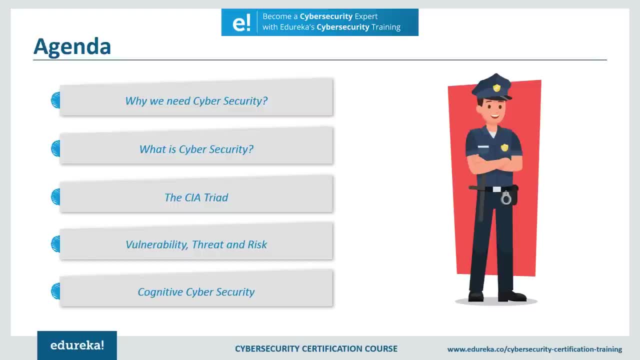 cyber security. Firstly, we're going to see why cyber security is needed. Next, we're going to see what exactly is cyber security and in the end, I'm going to show you all, through a scenario, how cyber security can save a whole organization from organized cyber crime. Okay, so let's get started. 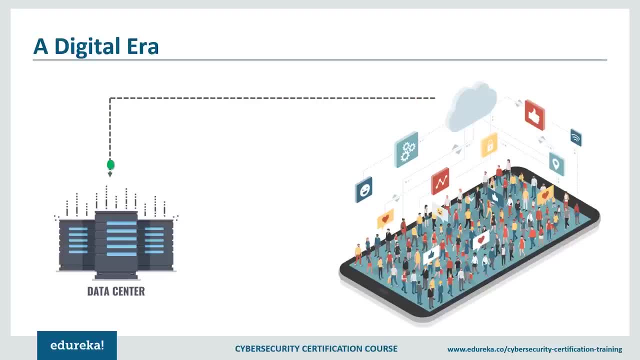 Now, as I just said, we are living in a digital era. Whether it be booking a hotel room, ordering some dinner or even booking a cab, we're constantly using the internet and, inherently, constantly generating data. This data is generally stored on the cloud, which is basically a huge 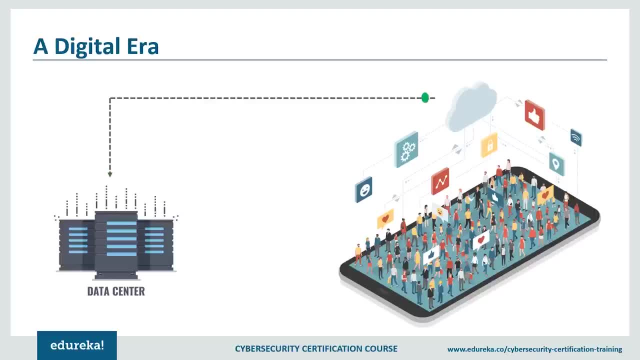 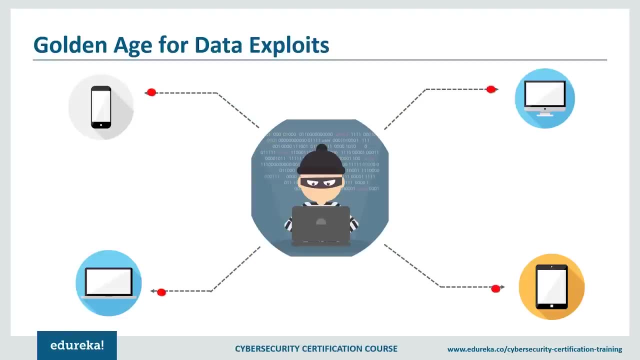 data server or data center that you can access online. Also, we use an array of devices to access this data. Now, for a hacker, it's a golden age, With so many access points, public IP addresses and constant traffic and tons of data to exploit. black hat hackers are having one hell of a time. 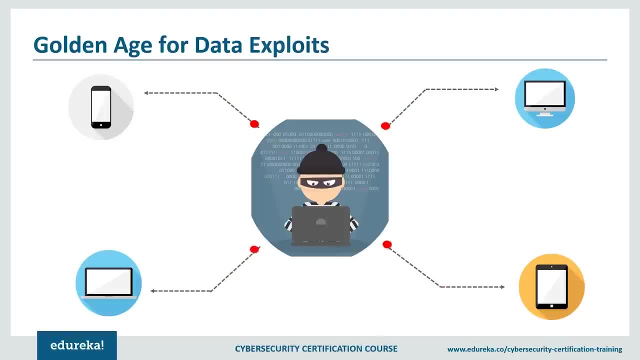 exploiting vulnerabilities and creating problems. So let's get started And creating malicious software for the same. Above that, cyber attacks are evolving by the day. Hackers are becoming smarter and more creative with their malwares, and how they bypass virus scans and firewalls still baffle many people. Let's go through some of the most common types. 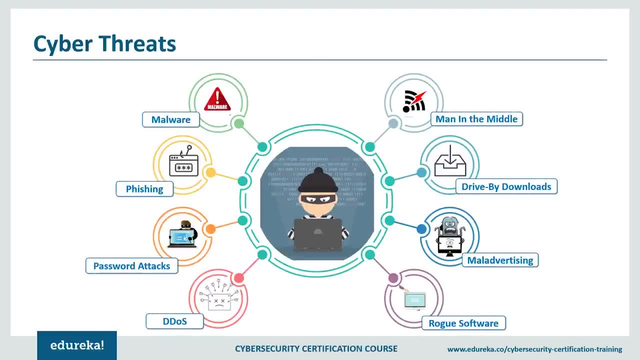 of cyber attacks now. So, as you guys can see, I've listed out eight cyber attacks that have plagued us since the beginning of the internet. Let's go through them briefly. So first on the list we have general malwares. Malware is an all-encompassing term for a variety of cyber threats. 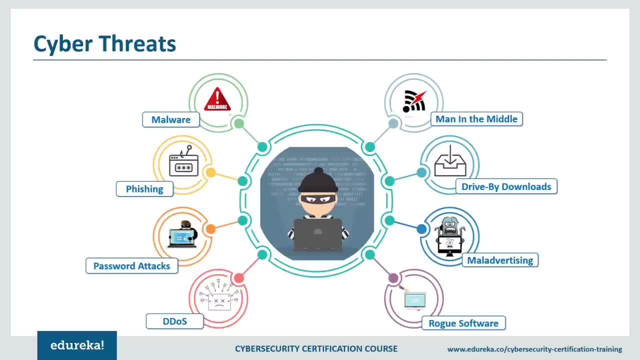 including Trojans, viruses and bombs. Malware is simply defined as code with malicious intent that typically steals data or destroys something on the computer. Next on the list we have phishing. Often posing as a request for data from a trusted third party, phishing attacks are sent via email. 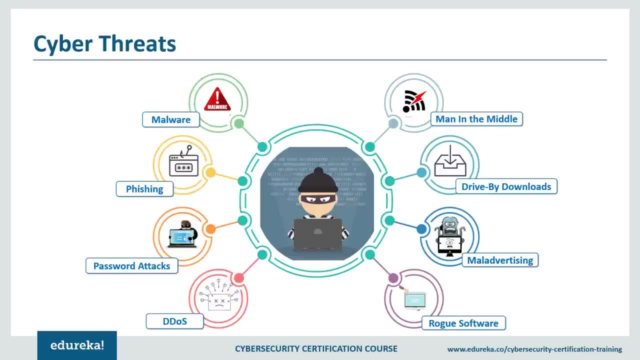 and ask users to click on a link and enter their personal data. Phishing emails have gotten much more sophisticated in recent years, making it difficult for some people to discern a legitimate request for information from a false one. Phishing attacks are often used to send a message to a. 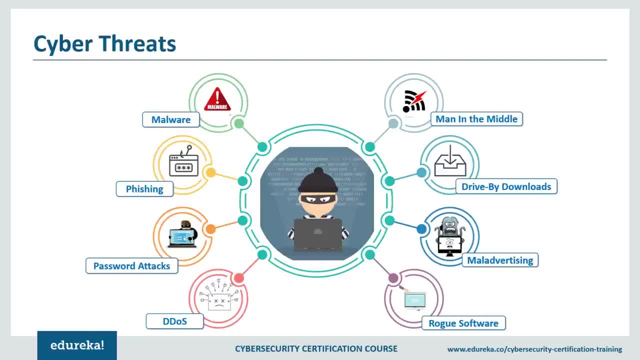 user. Phishing emails often fall into the same category as spam, but are more harmful than just a simple ad. Next on the list we have password attacks. A password attack is exactly what it sounds like: A third party trying to gain access to your system by cracking a user's password. 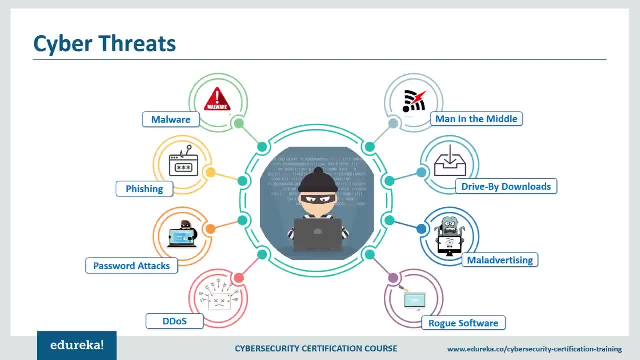 Next up is DDoS, which stands for distributed denial of service. A DOS attack focuses on disrupting the service of a network. Attackers send high volumes of data or traffic through the network. that is making a lot of connection requests Until the network becomes overloaded. 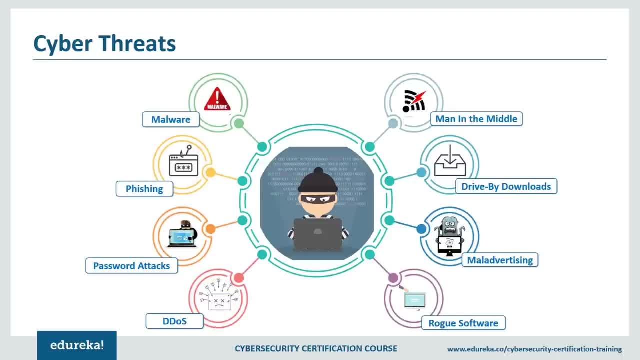 and can no longer function. Next up, we have man in the middle. attacks By impersonating the endpoint in an online information exchange. that is the connection from your smartphone to a website. the MITM attacks can obtain information from the end users and entity he or she is communicating. 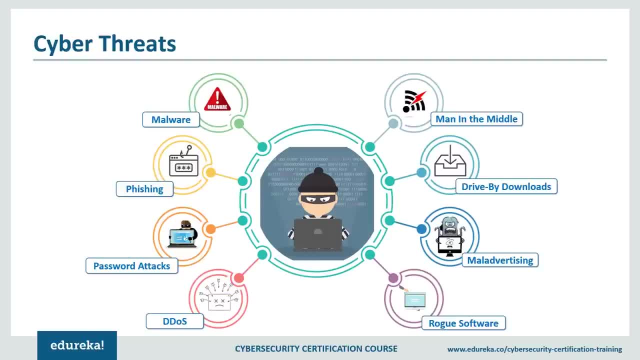 with. For example, if you're banking online, the man in the middle would communicate with you by impersonating your bank and communicate with the bank by impersonating you. The man in the middle would then receive all the information transferred between both parties and the. 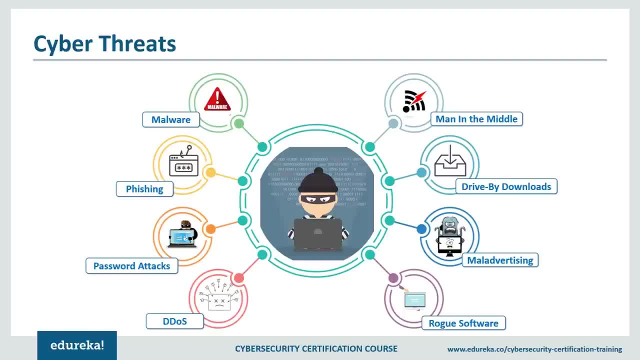 man in the middle would then receive more information, which could include sensitive data such as bank accounts and personal information. Next up, we have drive-by downloads Through malware. on a legitimate website, a program is downloaded to a user's system just by visiting the site. It doesn't require any type of action by the user to download it. actually, 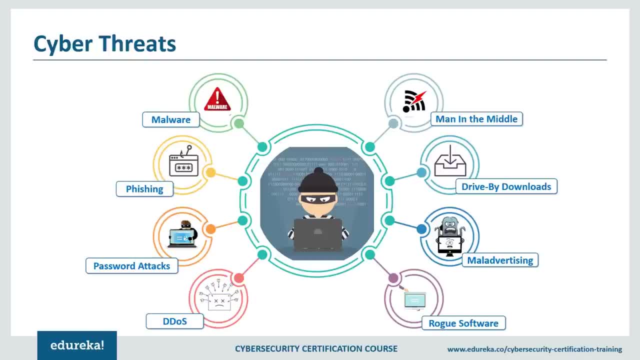 Next up, we have mal-advertising, which is a way to compromise your computer with malicious code that is downloaded to your system when you click on an affected ad. Lastly, we have rogue softwares, which are basically malwares that are masquerading as 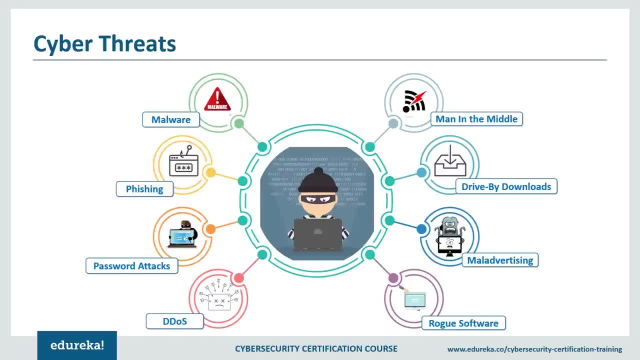 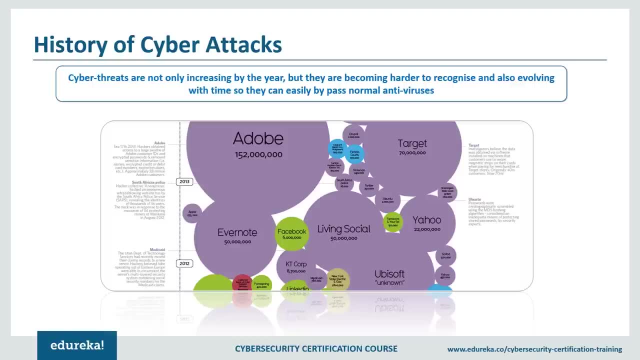 legitimate and necessary security software that will keep your system safe. So, as you guys can see now, the internet sure isn't a safe place as you might think it is. This not only applies for us as individuals, but also large organizations. There have been multiple cyber breaches in the past that has compromised the privacy. 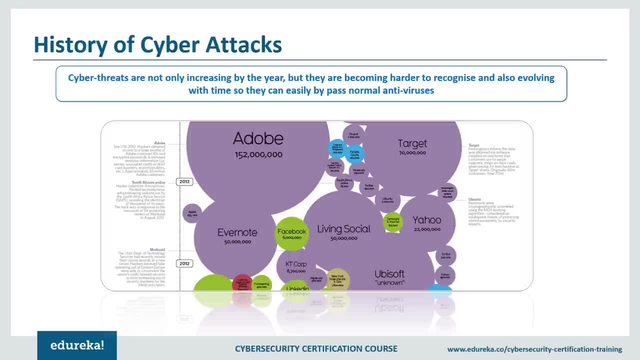 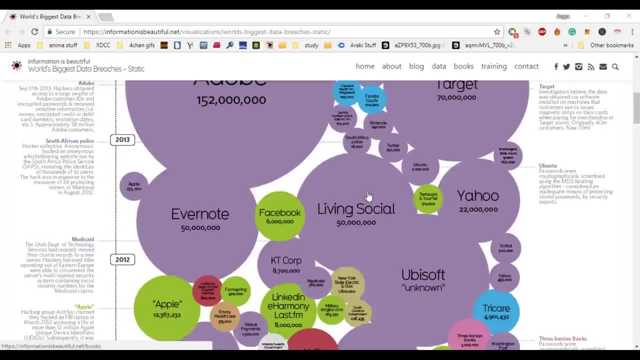 and confidentiality of our data. If we head over to the site called Information is Beautiful, we can see all the major cyber breaches that have been committed. So, as you guys can see, even big companies like eBay, AOL, Evernote, Adobe have actually 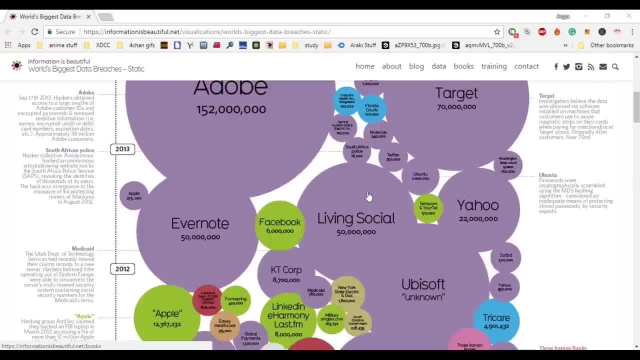 gone through major cyber breaches, even though they have a lot of security measures taken to protect the data that they contain. So it's not only that small individuals are targeted by hackers and other people, but even bigger organizations are constantly being targeted by these guys. 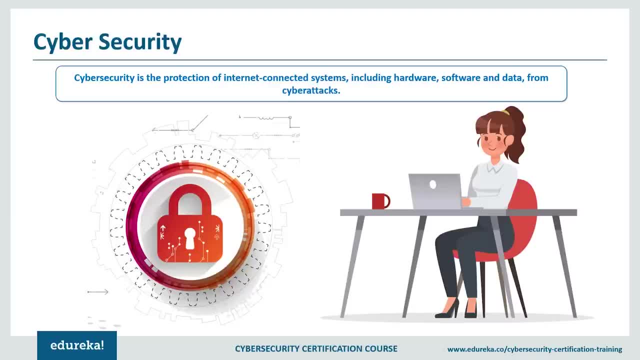 So, after looking at all sorts of cyber attacks possible, the breaches of the past and the sheer amount of data available, We must be thinking that there must be some sort of mechanism and protocol to actually protect us from all these sorts of cyber attacks. And indeed there is a way, and this is called cyber security. 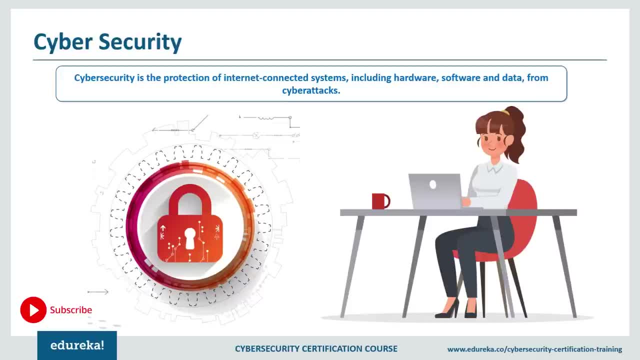 In a computing context, security comprises of cyber security and physical security. Both are used by enterprises to protect against unauthorized access to data centers and other computerized systems. Information security, which is designed to maintain the confidentiality, integrity and availability of data, is a subset of cyber security. 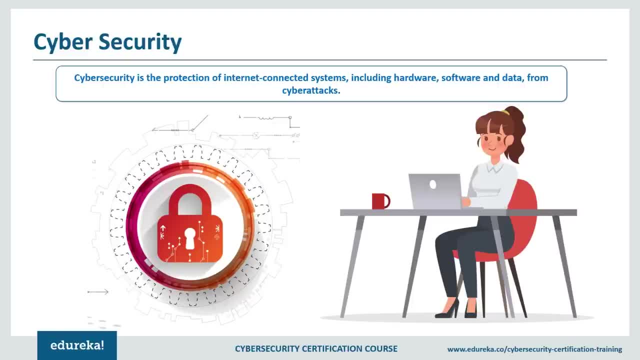 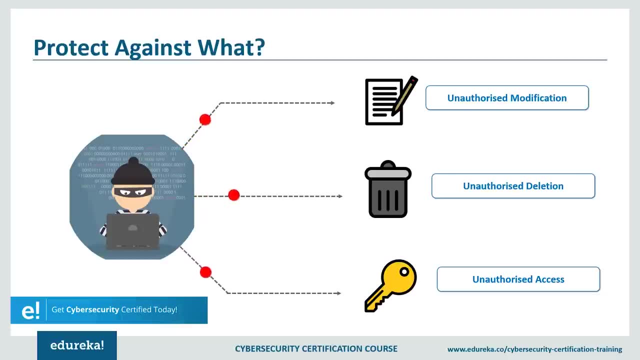 The use of cyber security is a very important part of data security. The use of cyber security is a very important part of data security. Security can help prevent against cyber attacks, data breaches, identity theft and can aid in risk management. So, when an organization has a strong sense of network security and an effective incident. 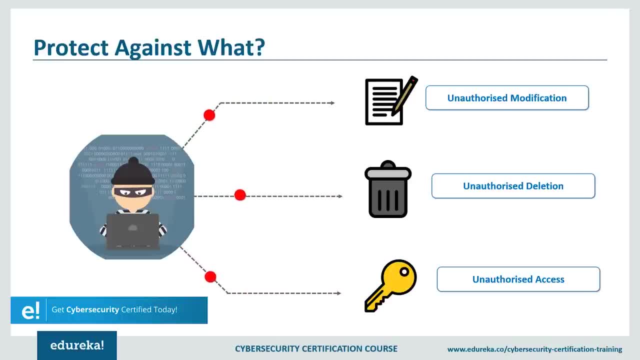 response plan. it is better able to prevent and mitigate these attacks, For example, end user protection, defense information and guards against loss of theft, while also scanning computers for malicious code. Now, when talking about cyber security, there are three main activities that we are trying. 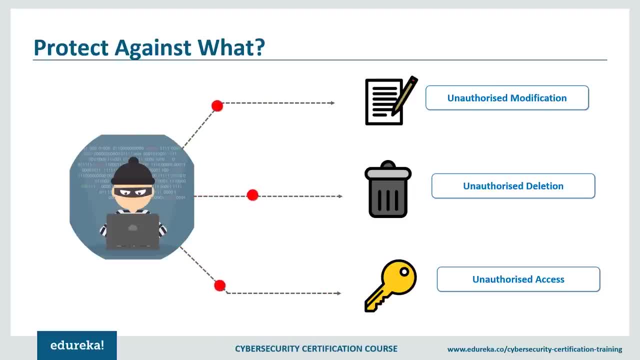 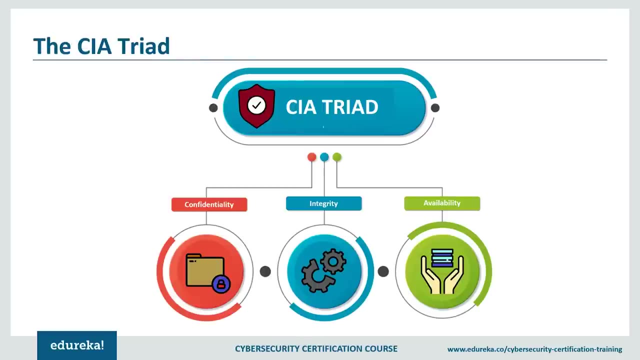 to protect ourselves against, And they are Unauthorized modification, unauthorized deletion and unauthorized access. These three terms are very synonymous to the very commonly known CIA triad, which stands for confidentiality, integrity and availability. The CIA triad is also commonly referred to as the three pillars of security. 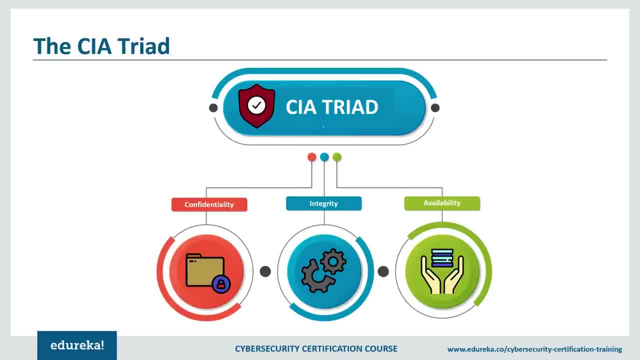 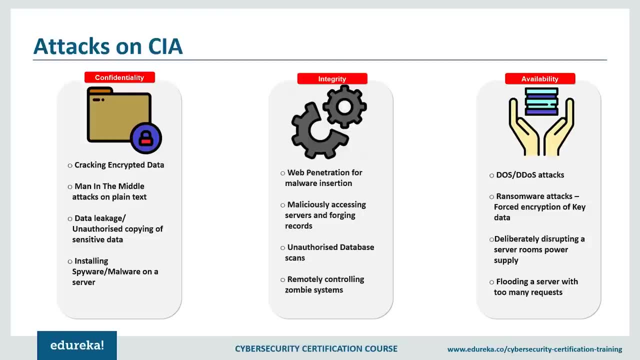 And most security policies of bigger organizations and even smaller companies are based on these three principles. So let's go through them one by one. So first on the list we have confidentiality. Confidentiality is roughly equivalent to privacy. Measures undertaken to ensure confidentiality are designed to prevent sensitive information. 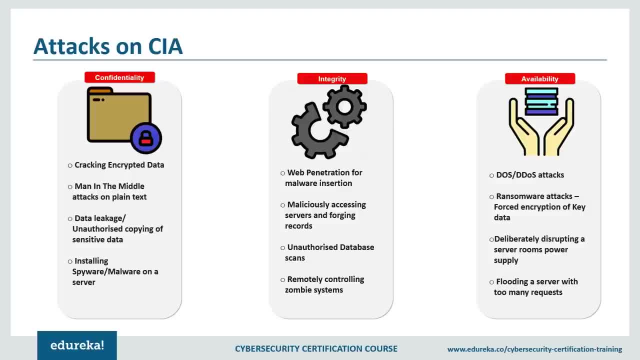 from reaching the wrong people, while making sure that the right people can in fact get it. Access must be restricted to those authorized to view the data in question. It is common as well for data to be categorized according to the amount and type of damage. 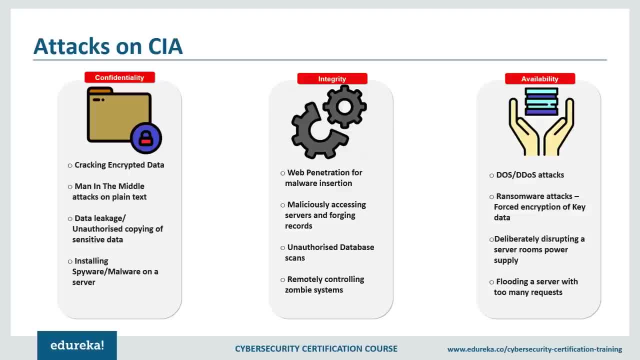 that could be done. should it fall into unintended hands, More or less stringent measures can then be implemented to protect the data. So let's look at some examples. The first is confidentiality. Confidentiality establishes the risk that a particular risk factors pose upon a particular 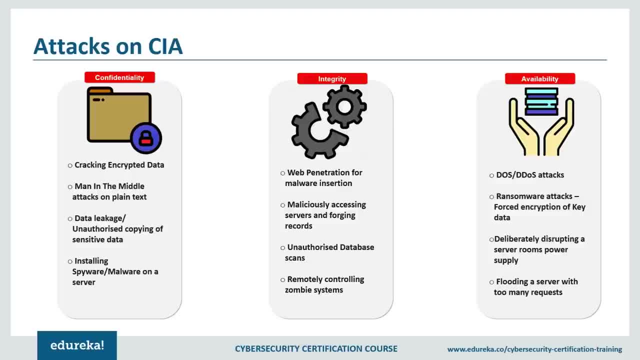 person. For example, a person's safety is a doctor's risk. A checkup may have to be made when a person attacks or storages a property. A person may not go to a hospital when he or she is diagnosed with a health risk. 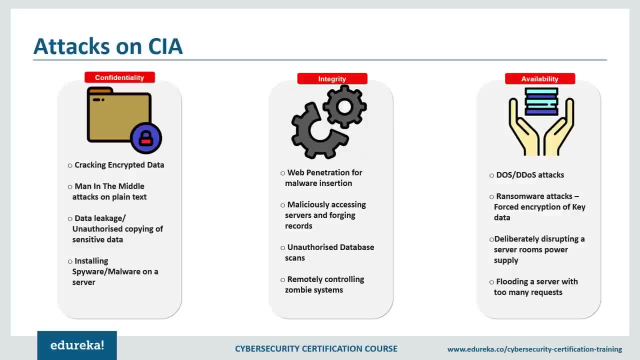 A person may go to see a doctor for a higher risk for mental illness. A person may go to a hospital for a minor or chronic illness. The second is confidentiality. Confidentiality can be used to protect individuals. A person may go to a health center or hospital for a SEARCH report. A person may go to a nurse or an emergency room. They may go to the doctor's office or the hospital to get a medical checkup. as a result of the behavior of the patient, They may go to a quieren center, where they may go to the hospital and they may get sent. 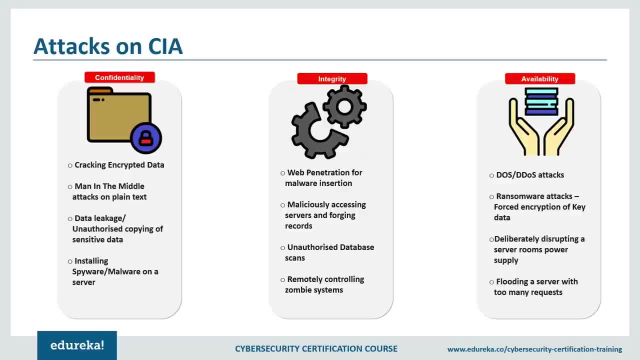 authorized people with risk factors and how to guard against them. Further aspects of training can include strong password and password-related best practices and information about social engineering methods to prevent them from bending data handling rules with good intention and potentially disastrous results. Next on the list we have integrity. Integrity involves maintaining 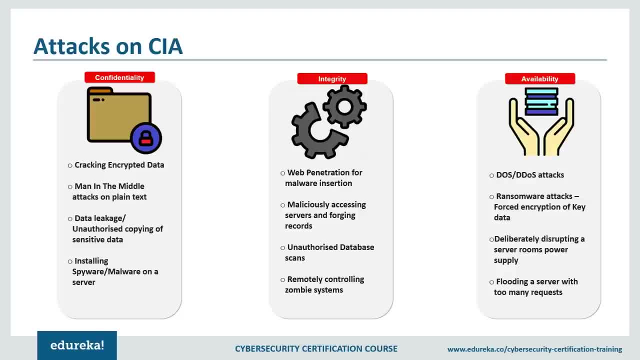 the consistency, accuracy and trustworthiness of data over its entire life cycle. Data must not be changed in transit and steps must be taken to ensure that data cannot be altered by unauthorized people, for example in a breach of confidentiality. These measures include file permissions and user. 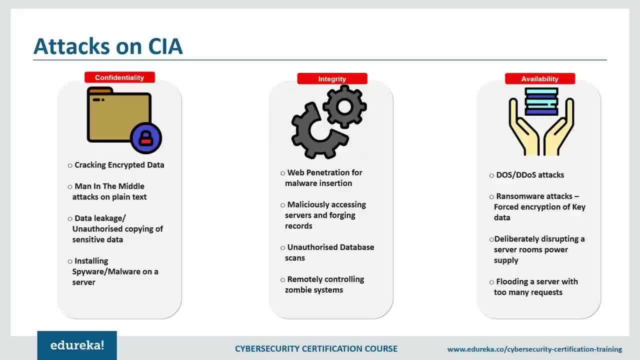 access controls. Version control may be used to prevent erroneous changes or accidental deletion by authorized users becoming a problem. In addition, some means must be in place to detect any changes in data that might occur as a result of non-human caused events, such as electromagnetic. 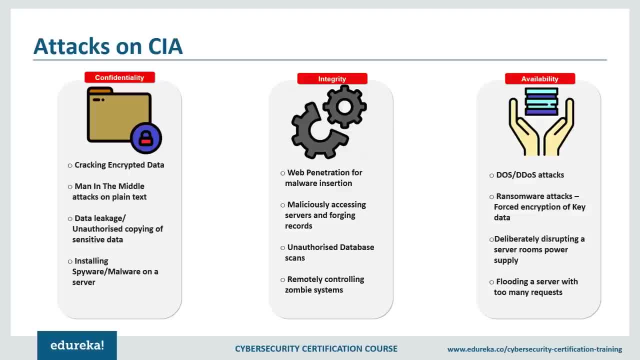 pulses or server crash. Some data might include checksums, even cryptographic checksums, for verification of integrity. Backup or redundancies must be available to restore the affected data to its correct state. Last but not least is availability. Availability is best ensured by rigorous maintaining of all 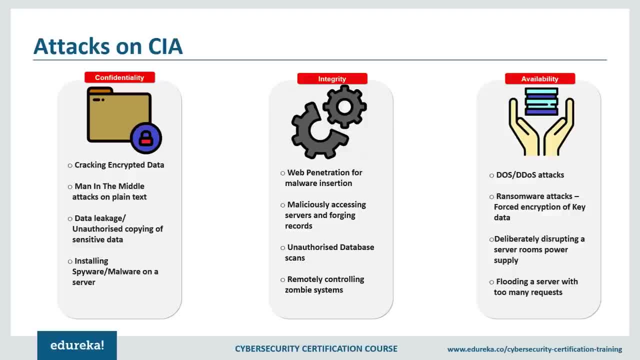 hardware, performing hardware repairs immediately when needed and maintaining a correctly functional operating system environment that is free of software conflicts. It is also important to keep current with all necessary system upgrades. Providing a secure system environment is a key factor for maintaining active communication with a user. 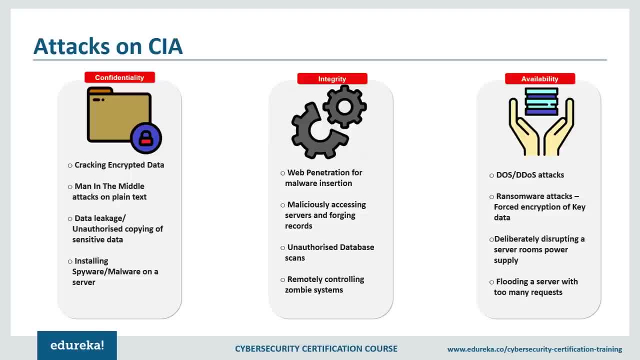 Providing adequate communication bandwidth and preventing the occurrences of bottlenecks are equally important. Redundancy, failover and even high availability clusters can mitigate serious consequences when hardware issues do occur. Fast and adaptive disaster recovery is essential for the worst-case scenarios. 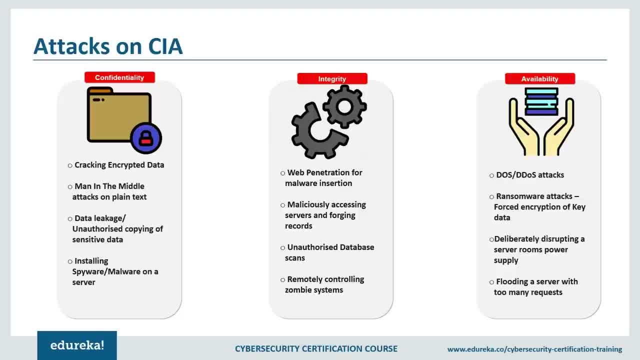 That capacity is reliant on the existence of a comprehensive disaster recovery plan. Safeguards against data loss or interruption in connection must include unpredictable events such as natural disasters and fire. To prevent data loss from such occurrences, a backup copy must be stored in a geographically 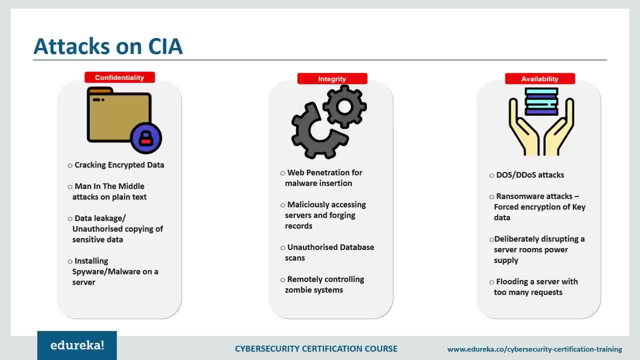 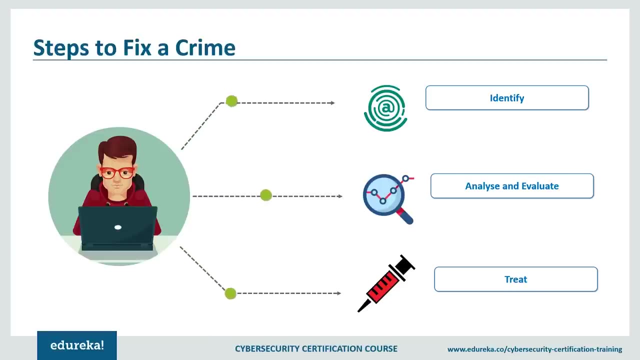 isolated location, perhaps even in a fireproof water safe place. Extra security equipments or software, such as firewalls and proxy servers, can guard us against downtimes and unreachable data due to malicious actions such as denial of service attacks and network intrusions. So, now that we have seen what we are actually trying to implement when trying to protect, 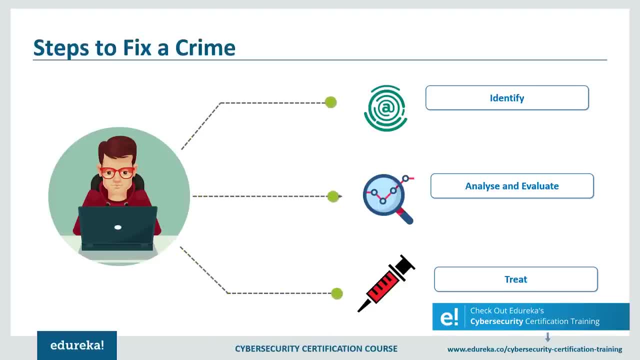 ourselves on the internet, We should also know The ways that we actually protect ourselves when we are attacked by cyber organizations. So the first step to actually mitigate any type of cyber attack is to identify the malware or the cyber threat that is being currently going on in your organization. 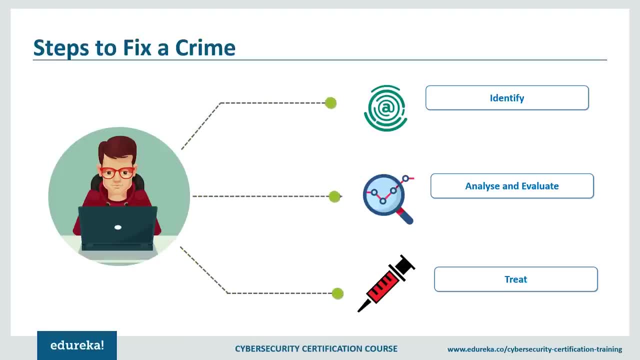 Next, we have to actually analyze and evaluate all the affected parties and the file systems that have been compromised And in the end, we have to patch the whole treatment so that our organization can come back to its original running state without any cyber breaches. So how is it exactly done? 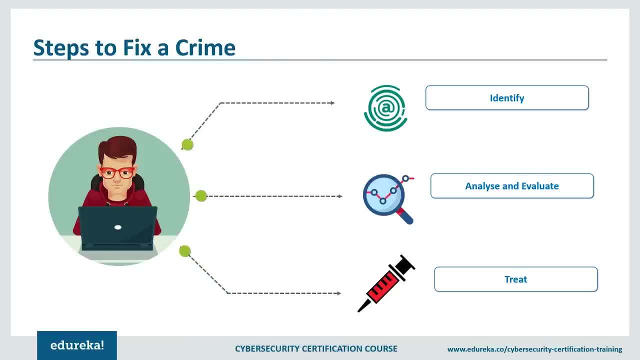 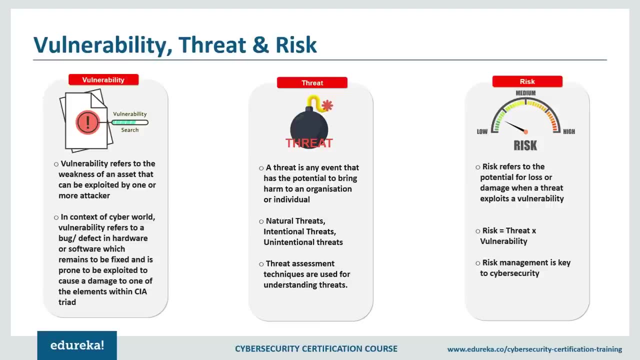 This is mostly done by actually calculating three factors. The first factor is vulnerability, The second factor is threat and the third is risk. So let me tell you about the three of them a little bit. So first, on the list of actual calculations, we have vulnerability. 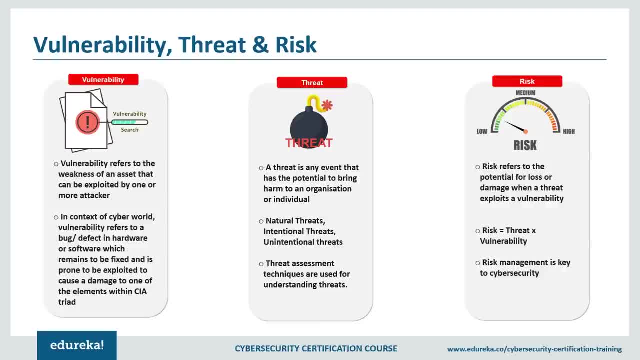 So a vulnerability refers to a known weakness of an asset that can be exploited by one or more attackers. In other words, it is a known issue that allows an attack to be successful, For example, when a team member resigns And you forget to disable their attack. 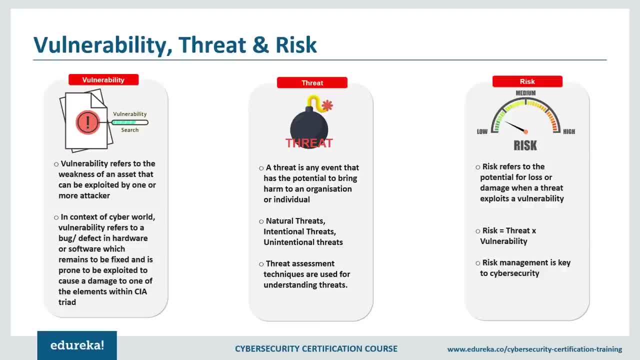 And you forget to disable their attack. If you change your access to external accounts, change logins or remove their names from the company credit cards, this leaves your business open to both unintentional and intentional threats. However, most vulnerabilities are exploited by automated attackers and not human typing. 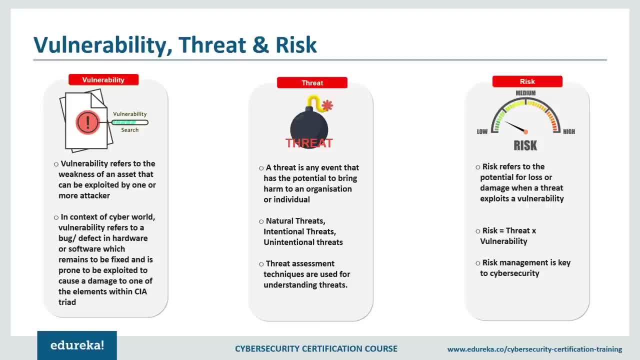 on the other side of the network. Next, testing for vulnerabilities is critical to ensuring the continued security of your systems by identifying weak points and developing a strategy to respond quickly. Here are some questions that you ask when determining a vulnerability. Number one is that: what is this vulnerability? 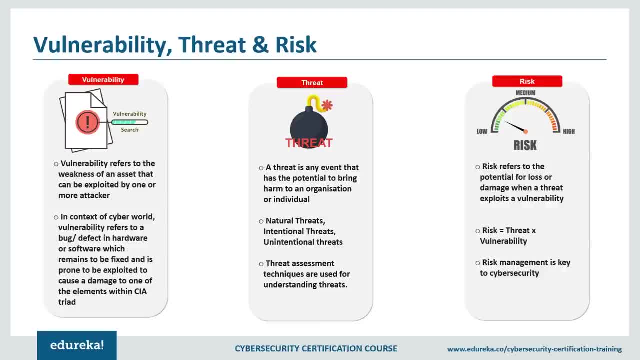 Number two is that: what is this vulnerability, your security vulnerabilities? so you have questions like: is your data backed up and stored in a secure off-site location? is your data stored in the cloud? if yes, how exactly is it being protected from cloud vulnerabilities? what kind of security do you have to determine who can access, modify or 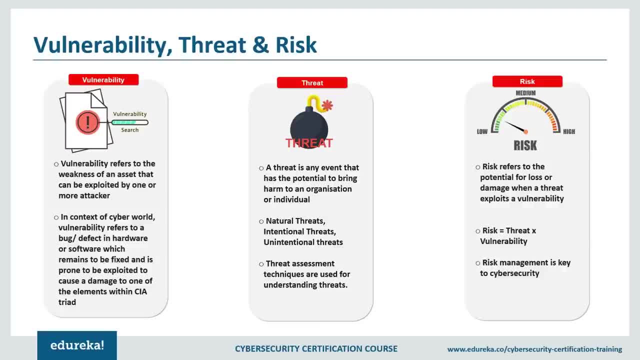 delete information from within your organization. next, like you could ask questions like: what kind of antivirus protection is in use? what are the license currents? are the license current and is it running as often as needed? also, do you have a data recovery plan in the event of vulnerability being? 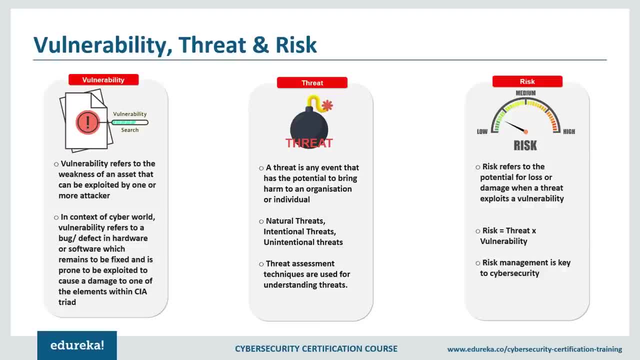 exploited? so these are the normal questions that one asks when actually checking their vulnerability. next up is threat. a threat refers to a new or newly discovered incident with potential to do harm to a system or your overall organization. there are three main types of threat: natural threats like floods, or 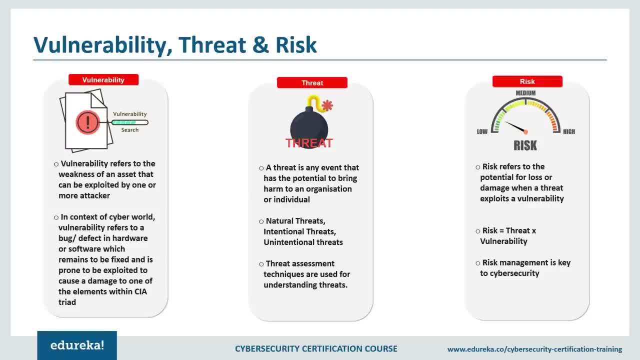 tornadoes, unintentional threats such as employee mistakenly accessing the wrong information, and intentional threats. there are many examples of intentional threats, including spyware, malware, adware companies or the actions of disgruntled employees. in addition, worms and viruses are categorized as threats because they could potentially cause harm to your 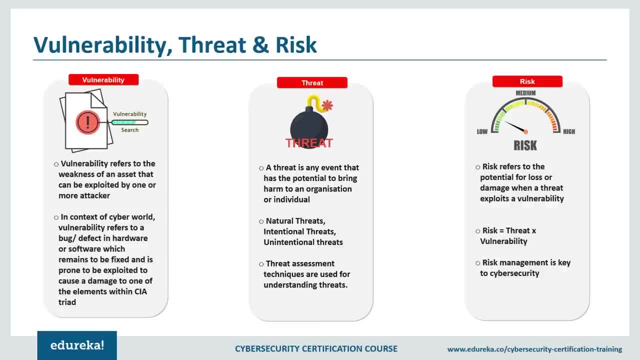 organization through exposure to an automated attack as opposed to one perpetrated by human beings. although these threats are generally outside of one's control and difficult to identify in advance, it is essential to take appropriate measures to assess threats regularly. here are some ways to do so: Ensure that your team members are staying informed of current trends in cyber. 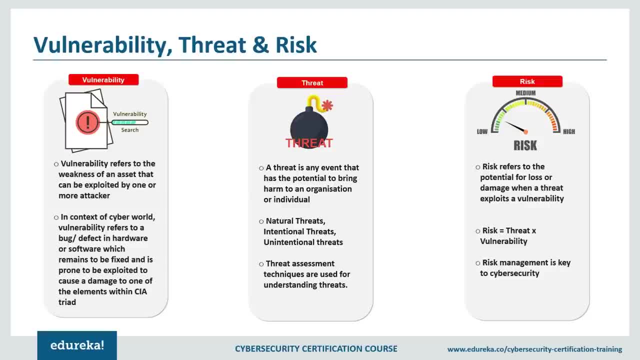 security so they can quickly identify new threats. They should subscribe to blogs like Wired and podcasts like the Techgenics Extreme IT that covers these issues, as well as join professional associations so they can benefit from breaking news feeds, conferences and webinars. You should 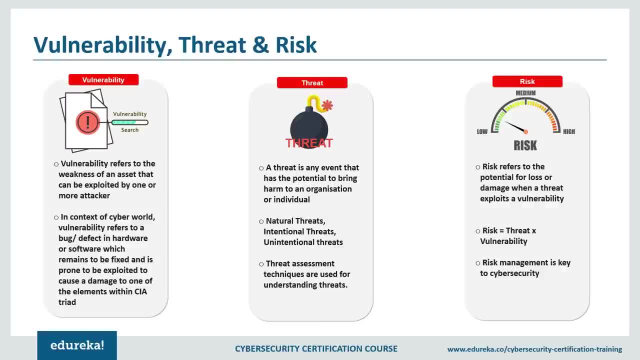 also perform regular threat assessment to determine the best approaches to protecting a system against a specific threat, along with assessing different types of threats. In addition, penetration testing involves modeling real-world threats in order to discover vulnerabilities. Next on the list we have risk. So risk refers to the potential for loss or damage when a threat 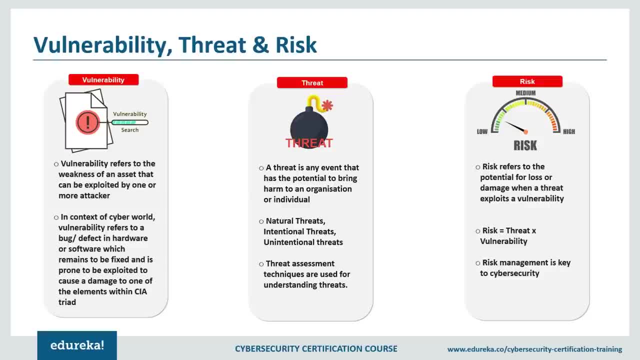 exploits a vulnerability. Examples of risks include financial losses as a result of business disruption, loss of privacy, reputational damage, legal implications, and can even include loss of life. Risk can also be defined as follows, which is basically threat multiplied by the vulnerability. You can reduce the potential for risk by creating 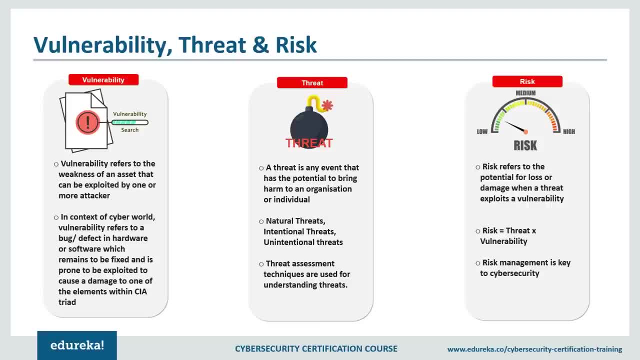 and implementing a risk management plan, and here are the key aspects to consider when developing your risk management strategy. Firstly, we need to assess risk and determine needs. When it comes to designing and implementing a risk assessment framework, it is critical to prioritize the most. 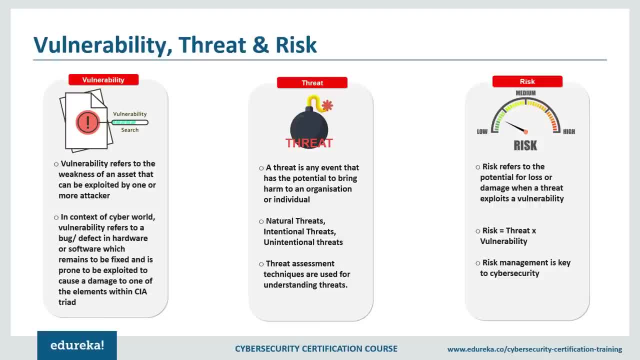 important breaches that need to be addressed. Although frequency may differ in each organization, this level of assessment must be done on a regular recurring basis. Next, we also have to include a total stakeholder perspective. Stakeholders include the business owners, as well as employees, customers and even vendors. All of these players have the potential to negatively. 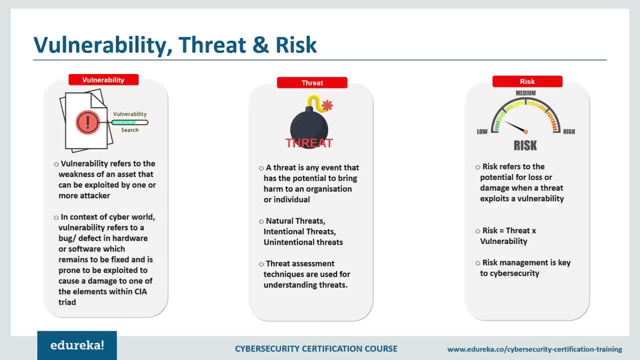 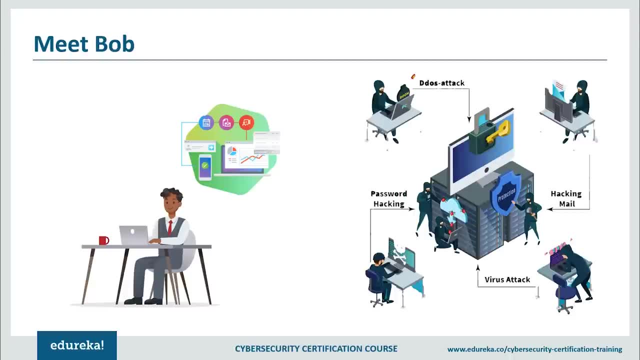 impact the organization, but at the same time, they can be assets in helping to mitigate risk. So, as we see, risk management is the key to cybersecurity. So now let's go through a scenario to actually understand how cybersecurity actually defends an organization against very manipulative 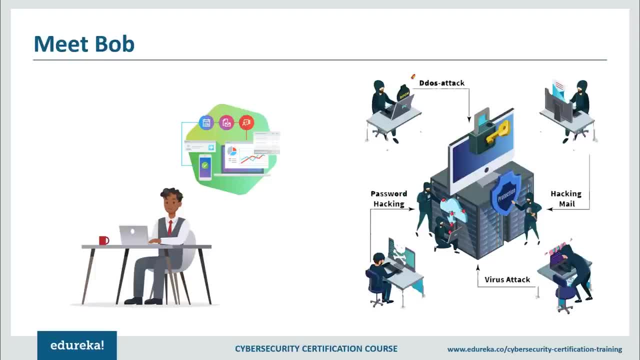 cybercrime. So cybercrime, as you all know, is a global threat. It's a very common threat to global problems that's been dominating the news cycle. It poses a threat to individual security and an even bigger threat to large international companies, banks and governments. Today's 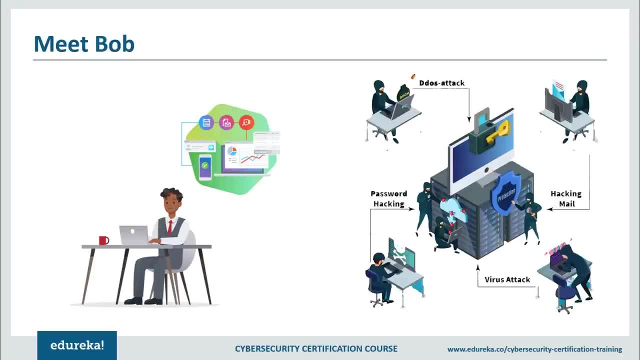 organized cybercrime far outshadows lone hackers of the past and now. large organized crime rings function like startups and often employ highly trained developers who are constantly innovating new online attack. Most companies have preventative security software to stop these types of attacks, but no matter how secure we are, cybercrime is going to happen. So meet Bob, He's the chief. 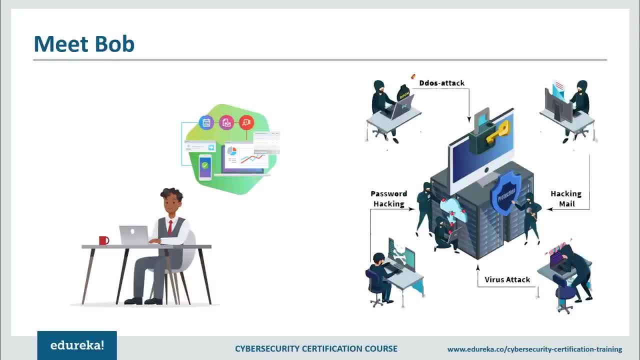 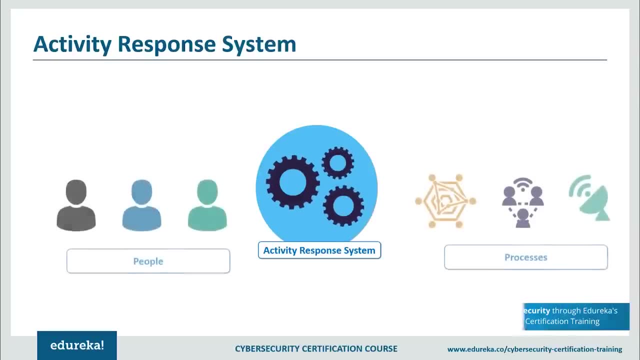 security officer for a company that makes a mobile app to help customers track and manage their finances. So security is a top priority. So Bob's company has an activity response platform in place that automates the entire cybersecurity process. The ARP software integrates all the security and 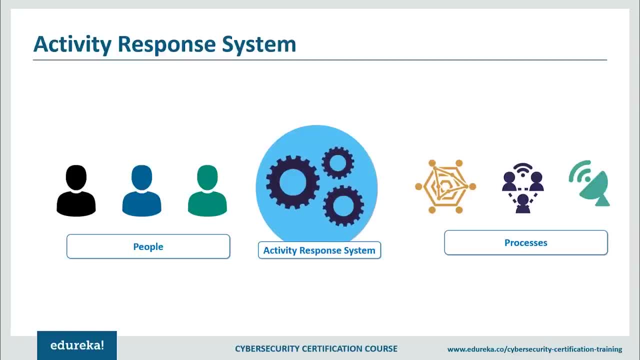 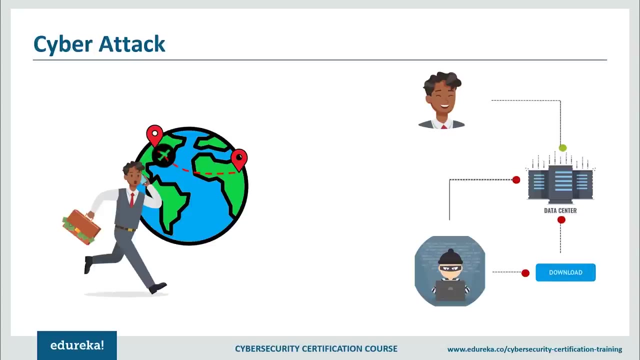 IT software needed to keep a large company like Bob's secure into a single dashboard and acts as a hub for the people, processes and technology needed to respond to and contain cyber attacks. Let's see how this platform works In the case of a security breach. while Bob is out on a business trip, irregular activity occurs. 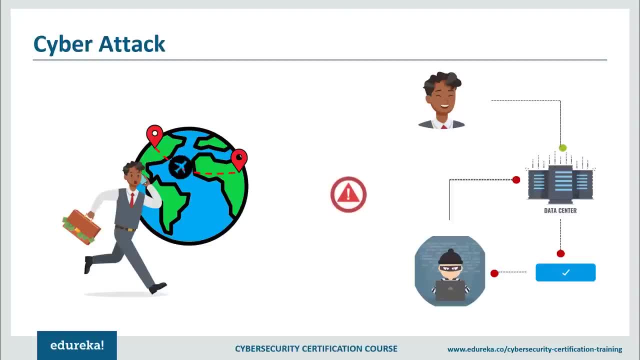 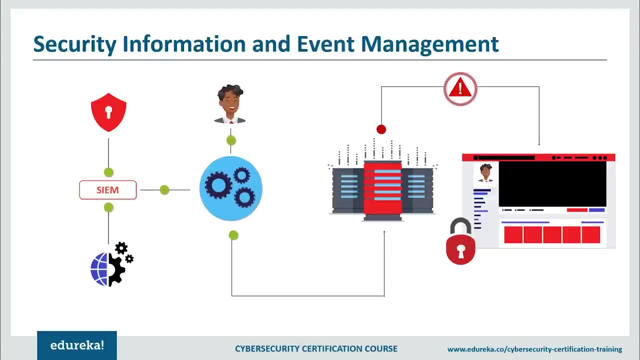 on his account as a user behavior analytics engine that monitors account activity recognizes suspicious behavior involving late night login and unusual amounts of data being downloaded. This piece of software is the first signal that something is wrong. An alert is sent to the next piece of software in the chain, which is the security information. 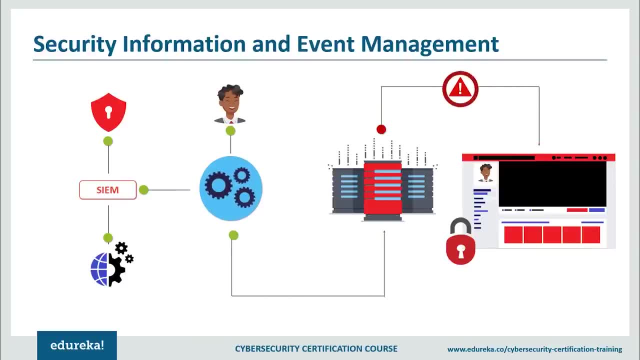 and event management system. Now the ARP can orchestrate a chain of of events that ultimately prevents the company from encountering a serious security disaster. The ARP connects to a user directory software that Bob's company uses, which immediately recognizes that user accounts belong to an executive who is out on a business trip and then proceeds to lock his. 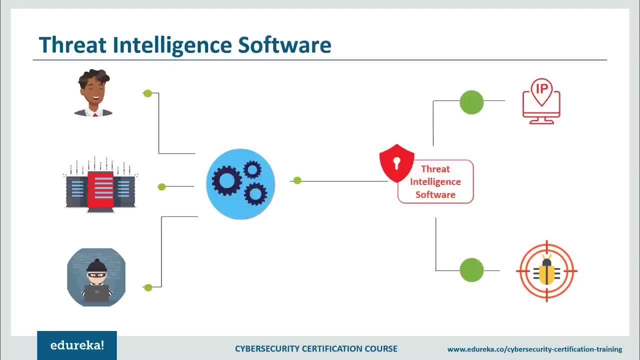 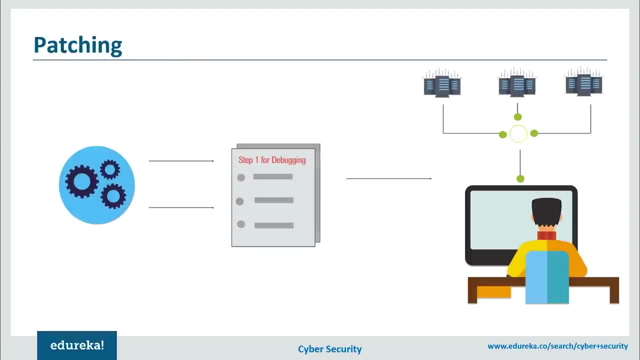 account, The ARP sends the incident IP address to a threat intelligence software which identifies the address as a suspected malware server. As each piece of security software runs, the findings are recorded in the ARP's incident, which is already busy creating a set of instructions called a playbook for a. 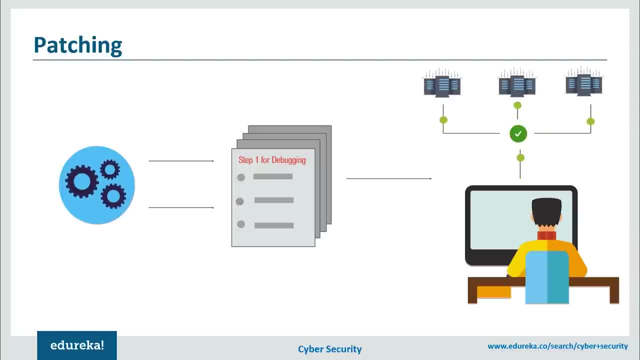 security analyst to follow. The analyst then locks Bob's accounts and changes his passwords. This time the software has determined the attempted attack came from a well-known cyber crime organization using stolen credentials. Bob's credentials were stolen when the hacker found a vulnerability in his 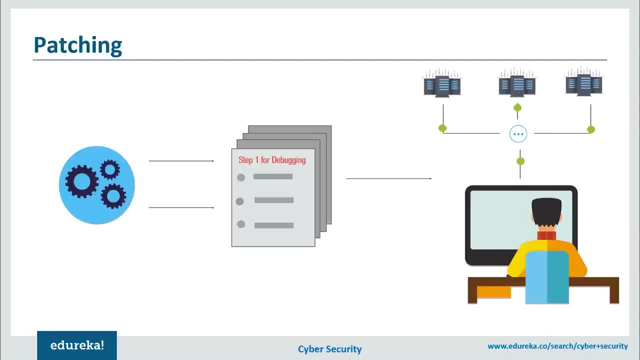 company's firewall software and used it to upload a malware infected file. Now that we know how the attack happened, the analyst uses the ARP and identifies and patches all the things. The ARP uses information from endpoint tool to determine which machines need to be patched. 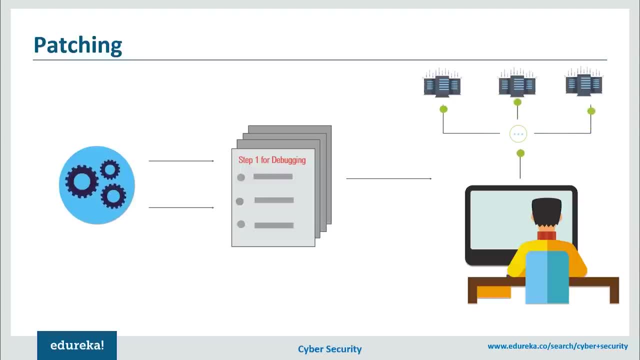 recommends how to patch them and then allows the analyst to push the patches to all the computers and mobile devices instantly. Meanwhile, Bob has to alert the legal departments of the breach and the ARP instantly notifies the correct person of the situation and the status of the incident after the attack is. 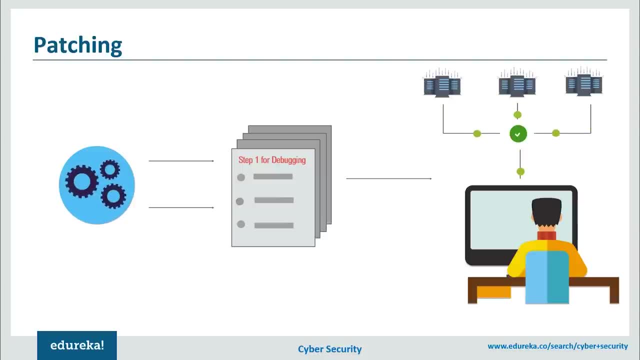 contained and Bob's account is secured. The analyst then communicates which data may have been stolen or compromised during the incident. He identifies which geographies, jurisdictions and regulatory agencies cover the users and information affected by the attack. Then the ARP creates a series of tasks so the organization can notify the affected parties.